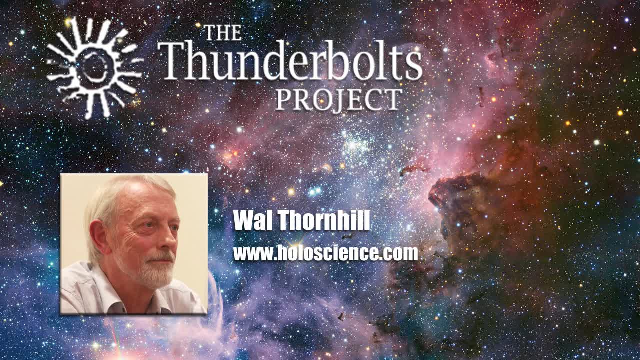 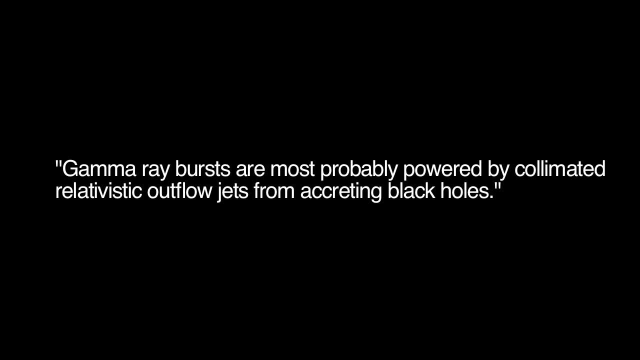 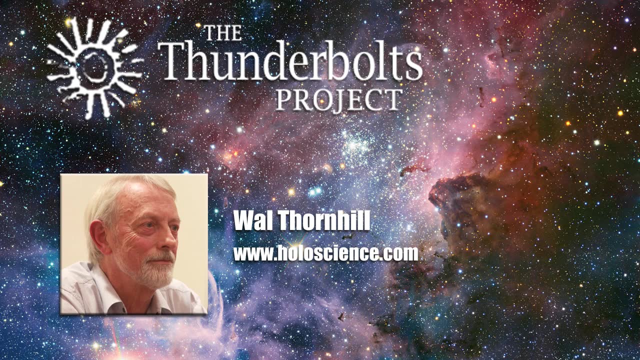 And this is borne out by the original Nature article that the Science News referred to where it starts: Gamma ray bursts are most probably powered by collimated relativistic outflow jets from accreting black holes. Well, as we've said repeatedly in the Space News, black holes do not exist. 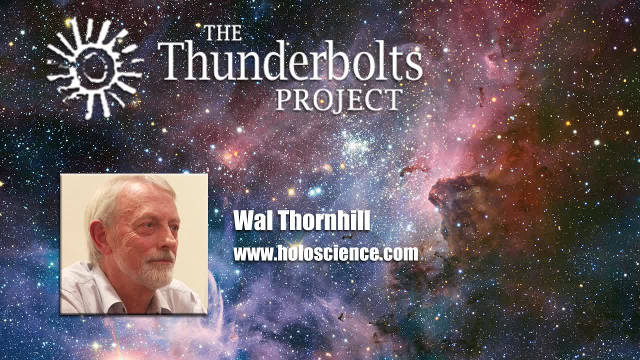 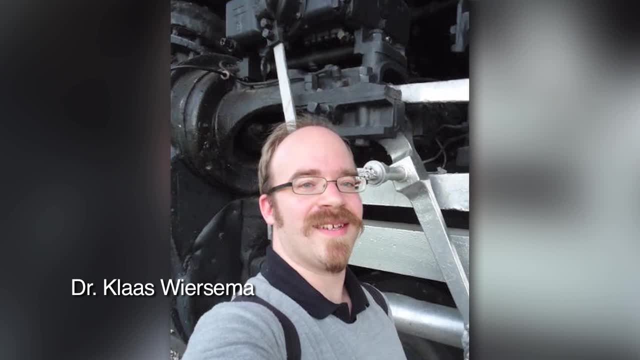 So it's not surprising that the findings that have just recently been discovered by Klaas Wiersma of the University of Leicester just don't match what they expected. In fact, the research itself is to be commended, because it was taking high precision. 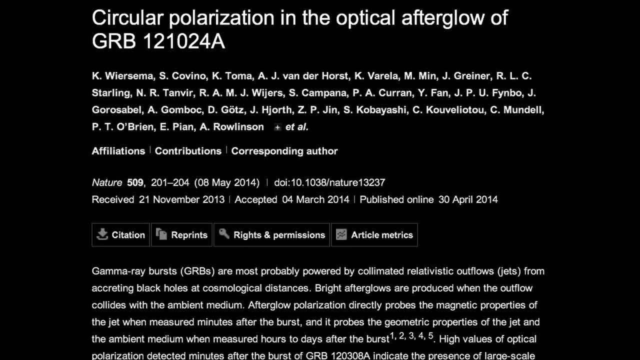 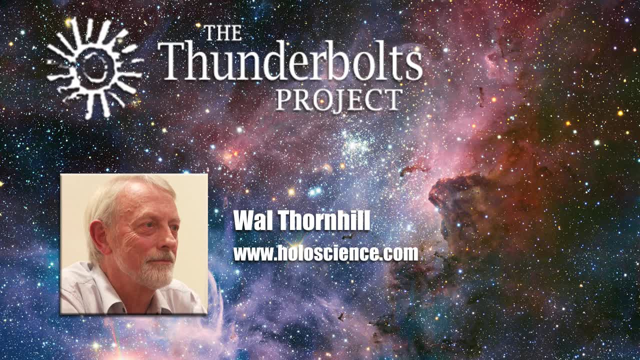 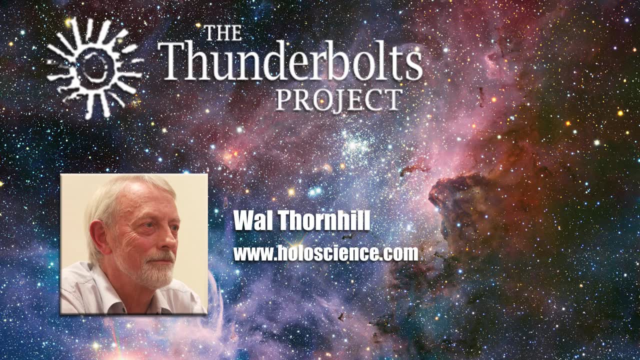 high precision measurements of a rapidly fading event in the sky, And it's very difficult from a technical point of view. So the research represents quite a technological achievement. The problem is that the findings were not expected at all. In fact, it was questioned why they would bother to do such an experiment. 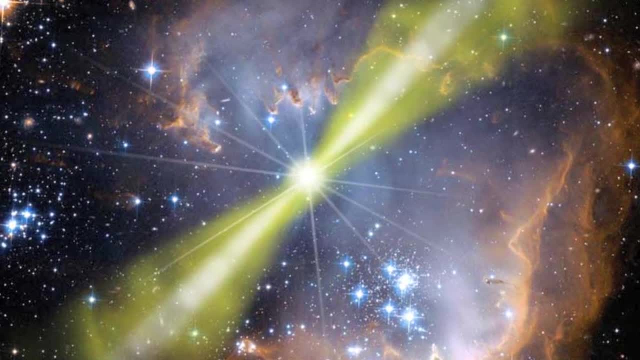 And that is to test the afterglow of a gamma ray burst to see what the polarization of the light was from that gamma ray burst. The Science News says that the gamma ray burst is the first time in the history of light. The Science News says that the gamma ray burst is the first time in the history of light. 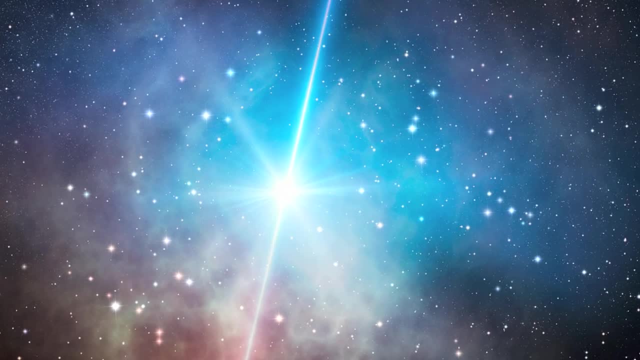 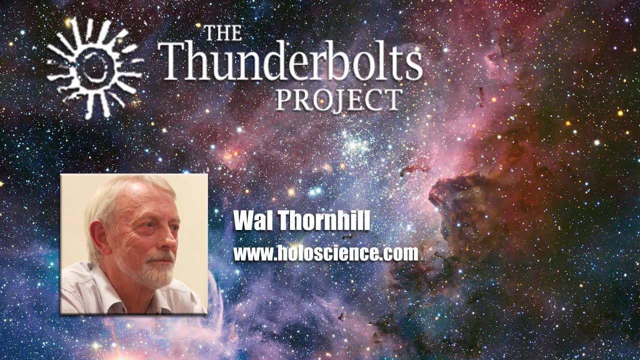 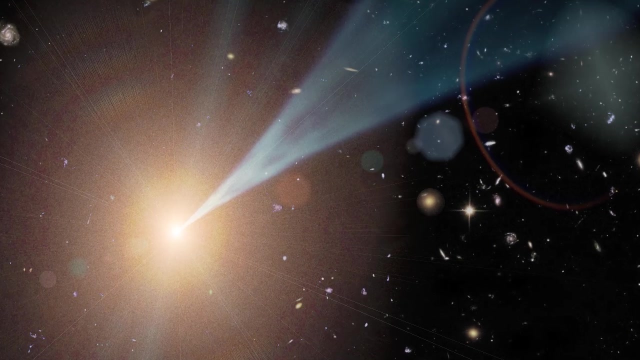 The Science News says that the gamma ray burst is one of the most powerful events in our universe. However, the discovery of polarization of the afterglow behaves completely differently than was previously thought. The new study published in Nature uses evidence from observations of a gamma ray burst. 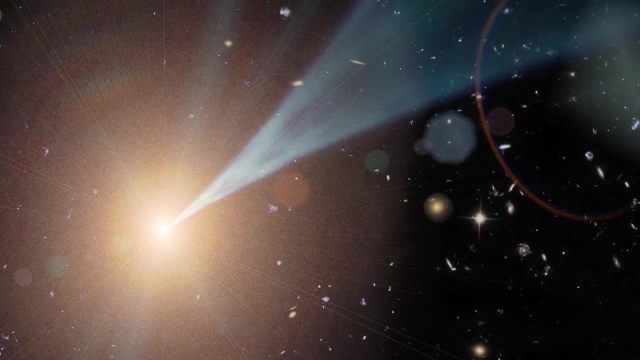 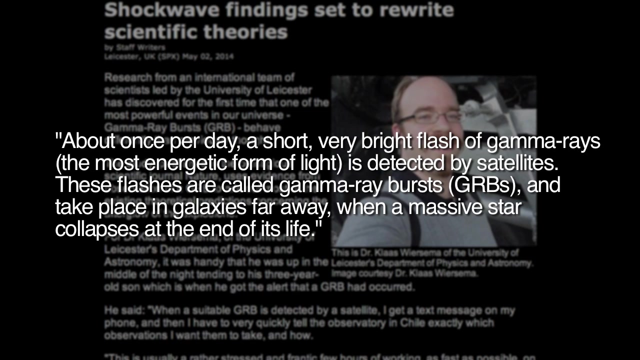 to rule out most of the existing theoretical predictions concerning the afterglow of such explosions. Dr Wiersma explains about once per day, a short, very bright flash of gamma rays- the most energetic form of light- is detected by satellites. These flashes are called gamma ray bursts and take place in galaxies far away. 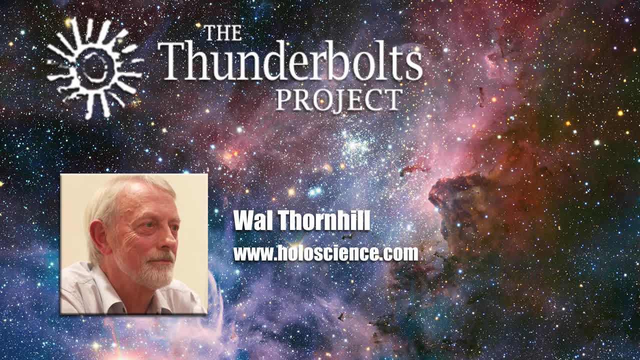 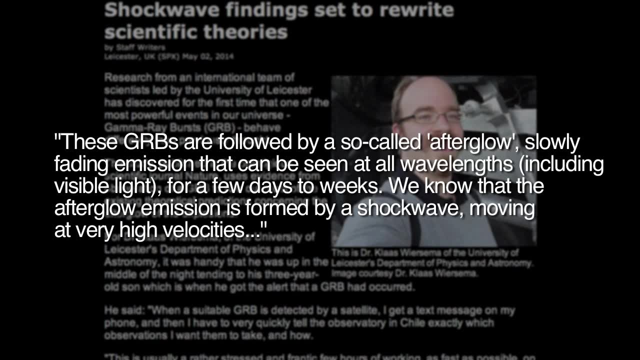 when a massive star collapses at the end of its life. Now, this is a statement of theoretical assumptions rather than a fact. These gamma ray bursts are followed by a so-called afterglow, a slowly fading emission that can be seen at all wavelengths, including invisible light. 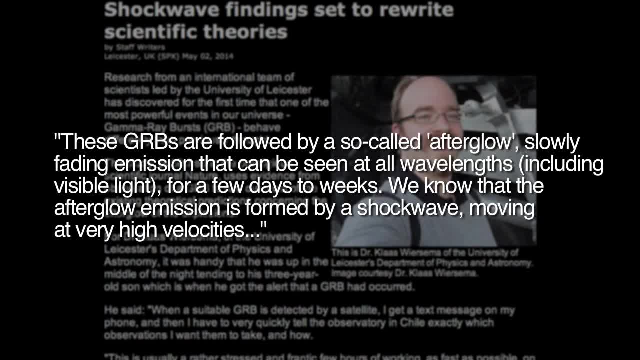 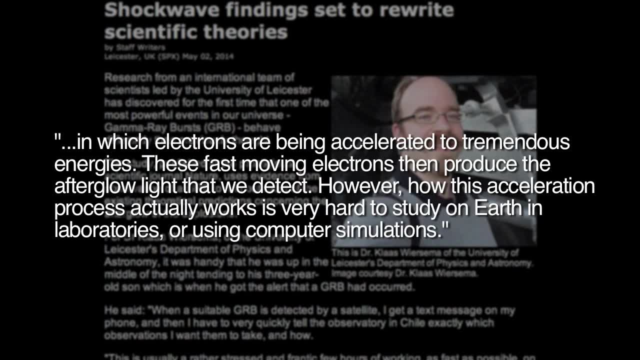 for a few days to weeks. We know that the afterglow emission is formed by a shock wave Moving at very high velocities, in which electrons are being accelerated to tremendous energies. These fast-moving electrons then produce the afterglow light that we detect. 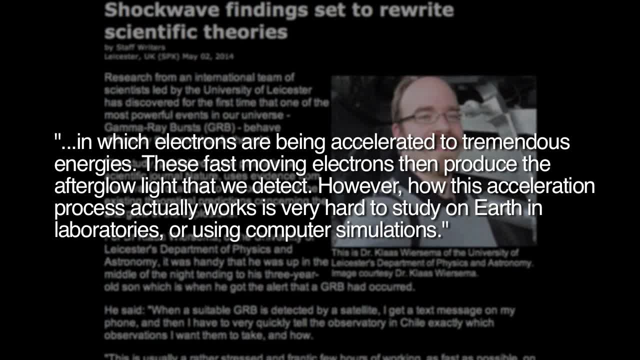 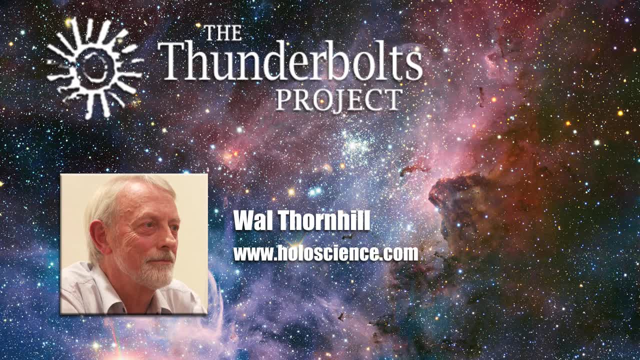 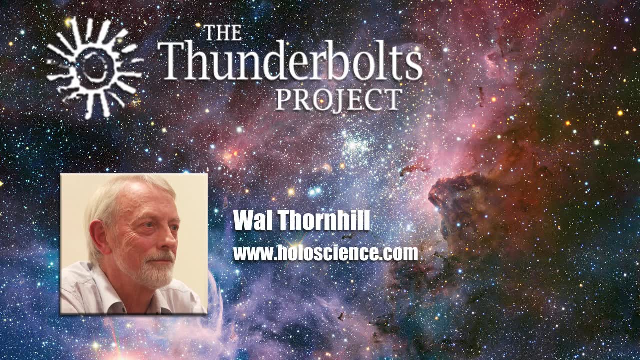 Dr Wiersma says. how this acceleration process actually works is very hard to study on Earth, in laboratories or using computer simulations. So what they did was to study the polarized light of the afterglow using large optical telescopes and special filters that work much like the filters in Polaroid sunglasses. 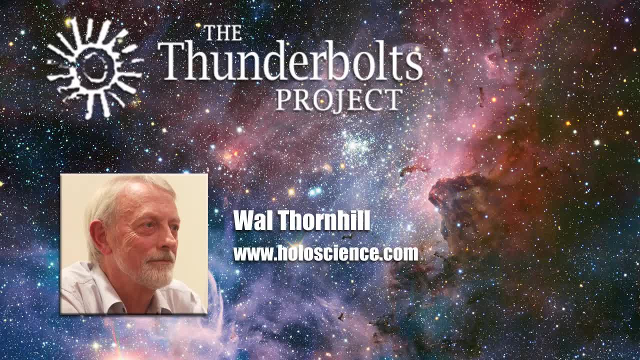 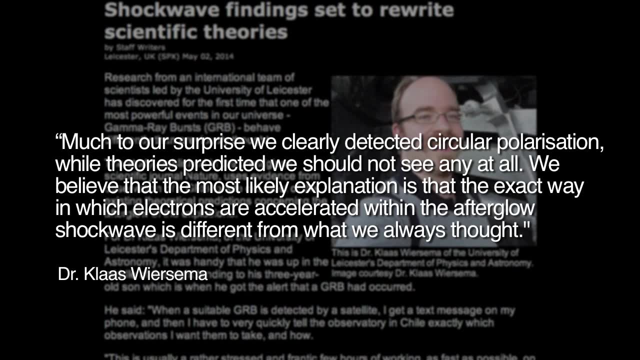 to detect the polarization of the light. Dr Wiersma goes on to say. much to our surprise, we clearly detected circular polarization, while theories predicted we should not see any at all. We believe that the most likely explanation is that the exact way in which electrons are accelerated 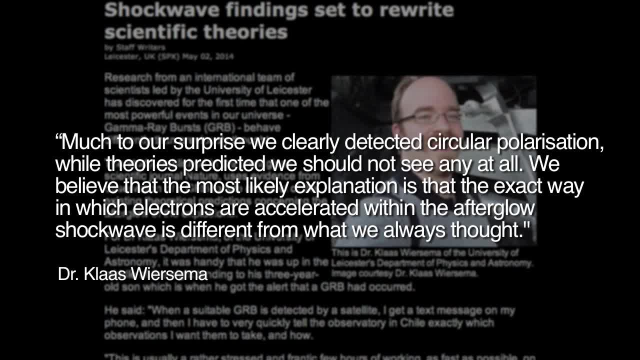 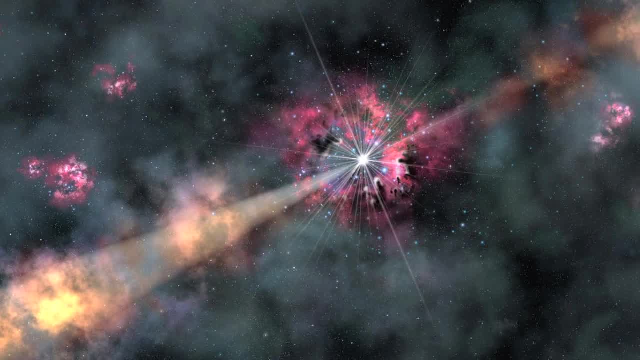 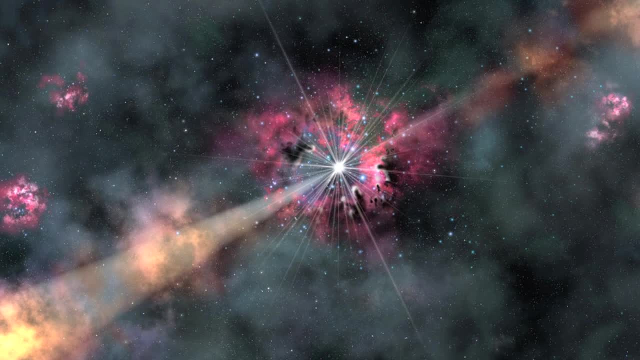 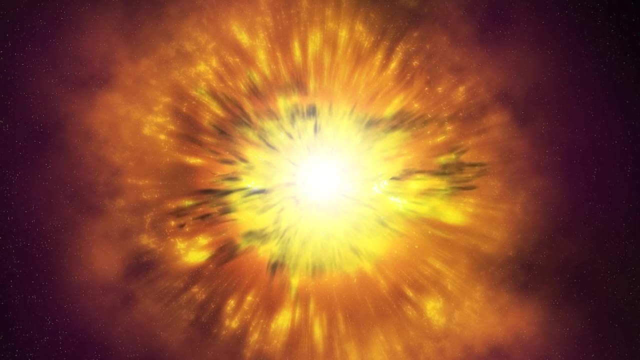 within the afterglow shock wave is different from what we always thought, And here we come to the Electric Universe model, because the gamma ray bursts are expected to be very high-energy electrical discharge events from the centers of active objects like quasars and stars that are suffering as a result of a supernova-type explosion. 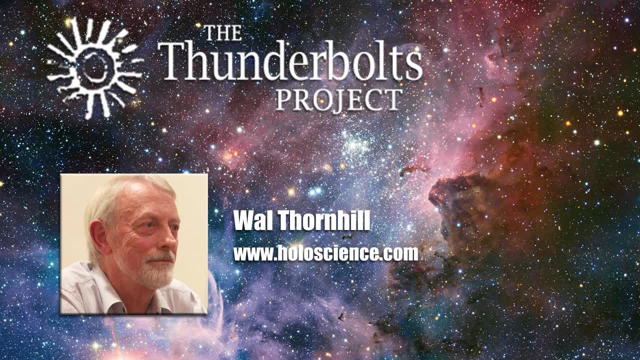 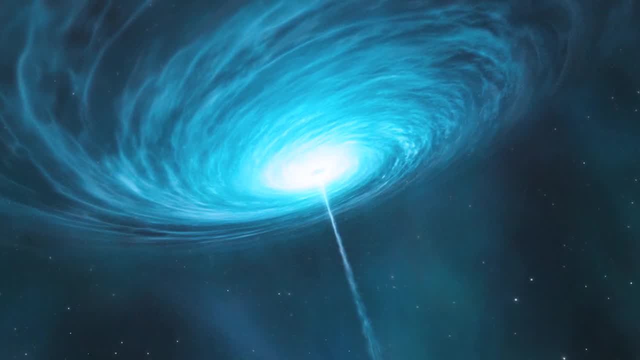 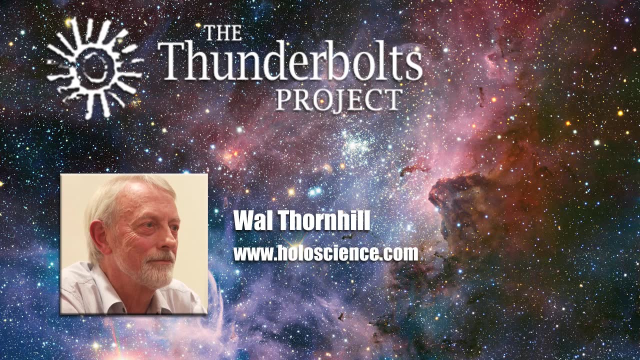 In both cases, the Electric Universe sees the object, the quasar or the supernova, as being the object in the center of a very active electrical discharge And therefore the origin of the radiation and so on is actually extended beyond the star and is part of a circuit. 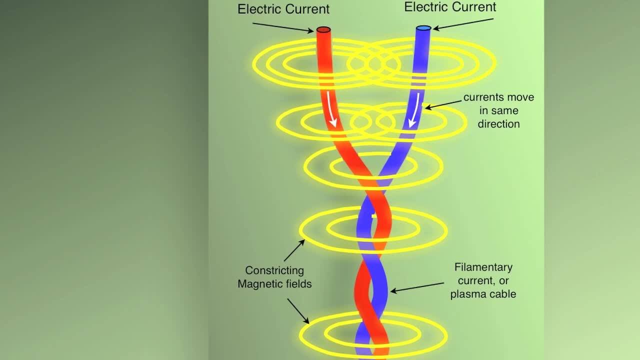 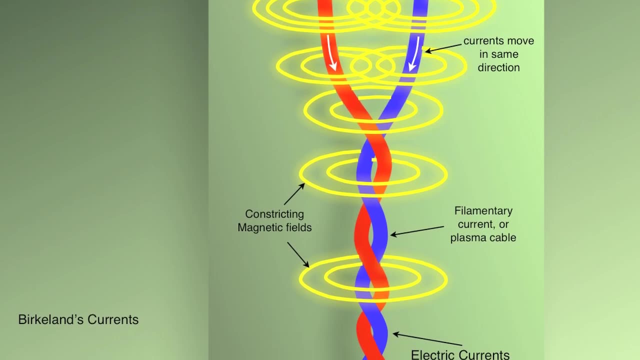 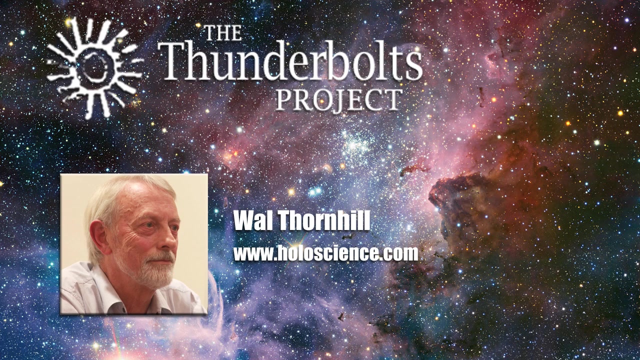 And these circuits are formed by Birkeland currents, And Birkeland currents have magnetic fields wrapped around them and the polarization of the electrons following those magnetic fields varies. in other words, it rotates and forms circular polarization. So this experiment actually confirms the Electric Universe model of a gamma ray burst. 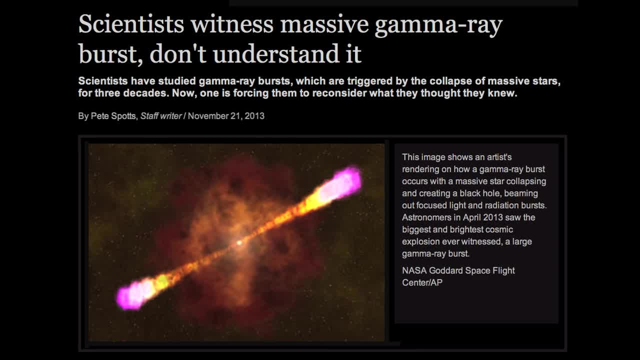 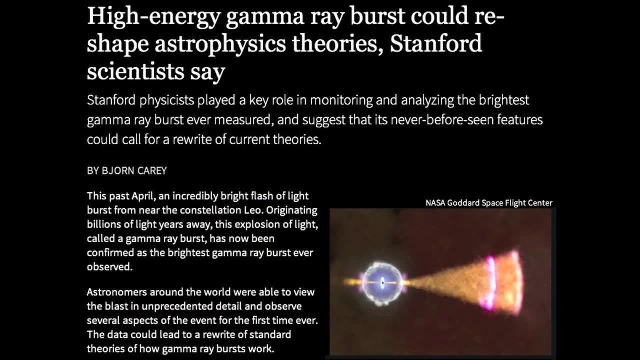 In late 2013,. astronomers around the world were astonished when a gamma ray burst was detected that lasted not a matter of mere milliseconds, but for an unprecedented 20 hours. Investigator Charles Dermer of Los Alamos National Laboratory said at the time: 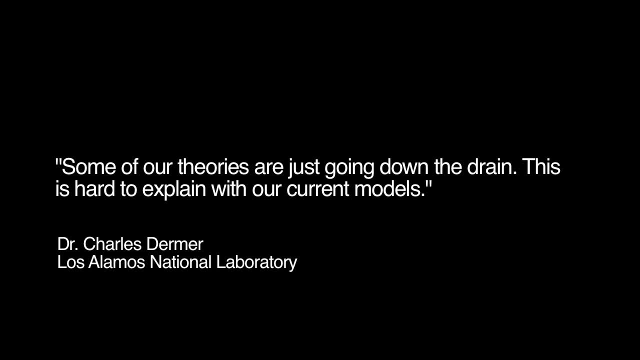 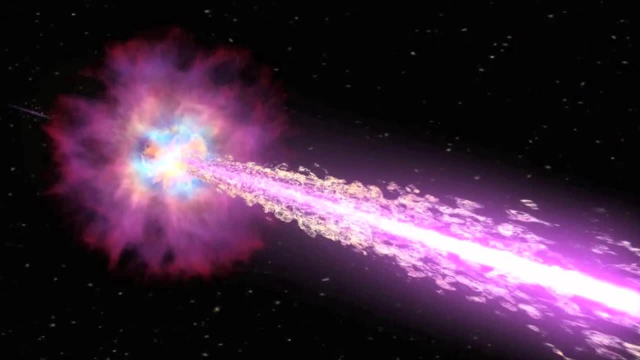 "some of our theories are just going down the drain. This is hard to explain with our current models". However, like this latest discovery, such an astonishing event may be reconciled with an electrical interpretation of gamma ray bursts. The Electric Universe is a Supernova. 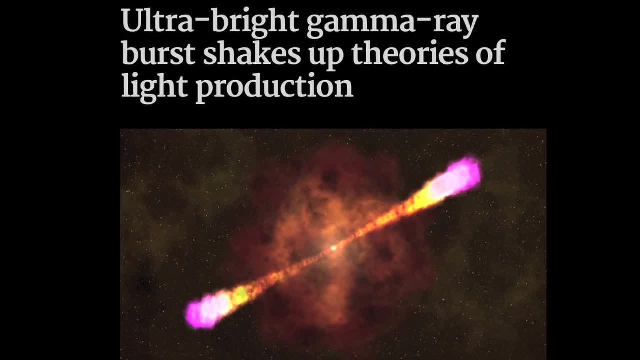 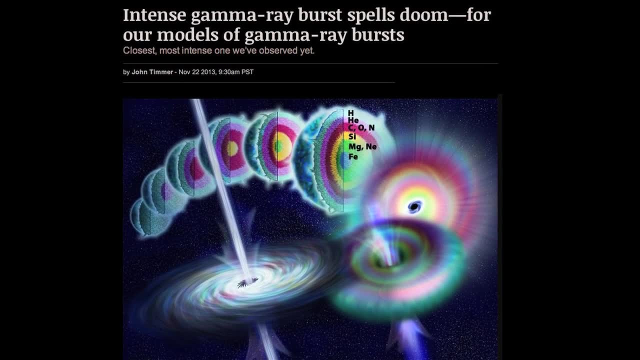 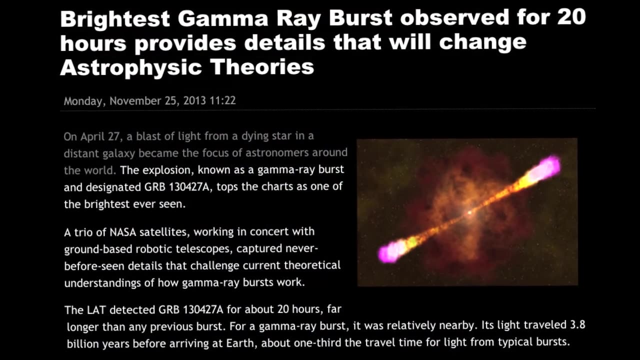 Some months ago, we reported on a gamma ray burst which lasted much longer than expected. Once again, the Electric Universe model expects this kind of thing, because the gamma ray burst is due to an extended electrical circuit And therefore the activity in that circuit can last much longer. 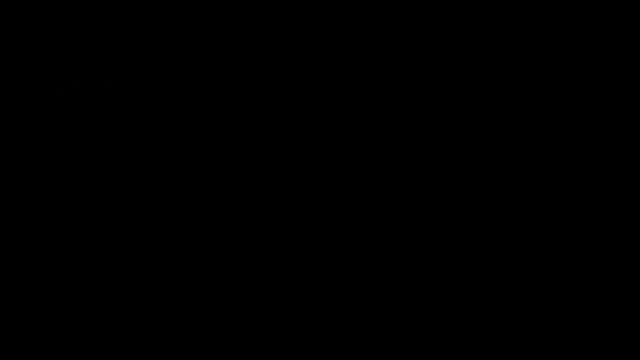 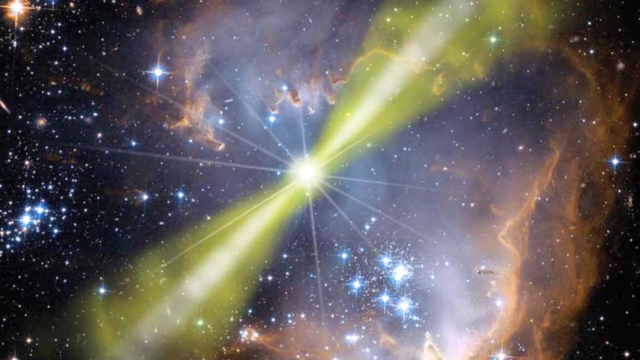 than something which is concentrated on a tiny star. The paper in Nature refers to the gamma ray burst as being due to shock waves- a collision by relativistic. due to shock waves. The gamma ray burst is due to a jet smashing into the surrounding matter. 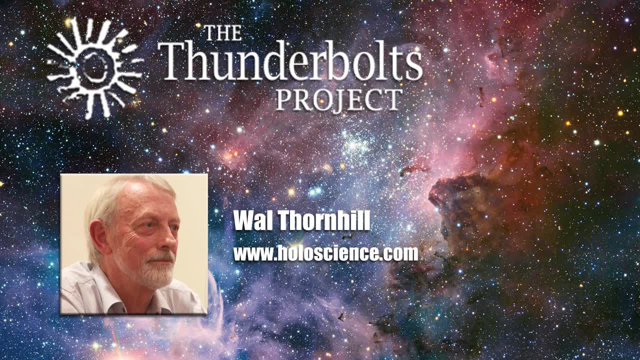 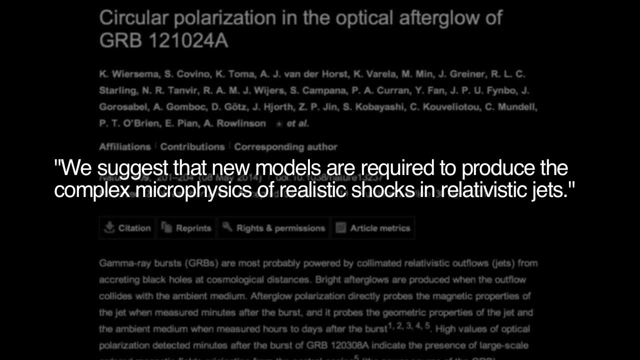 This makes all kinds of assumptions, of course, And in fact the article says: "we suggest that new models are required to produce the complex microphysics of realistic shocks in relativistic jets", But this raises the whole issue of whether such jets are the origins of these bursts. 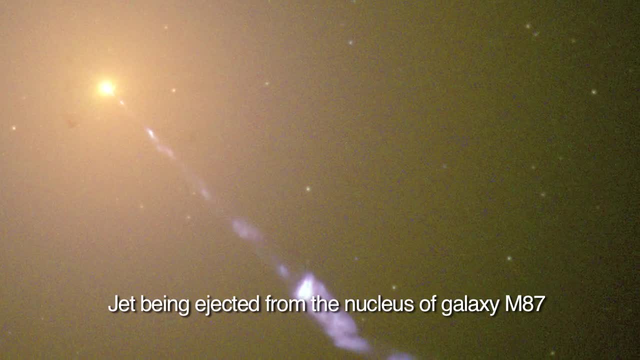 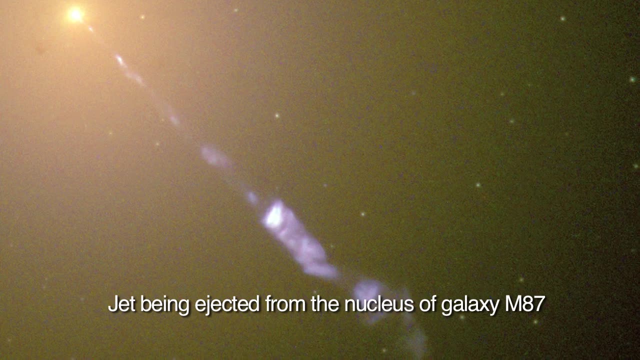 It's never been shown precisely how a jet can remain trained like a fire hose in a particular direction and not be diverted by matter in the path of that fire hose outburst, if you like. And this is where the Electric Universe model makes far more sense. 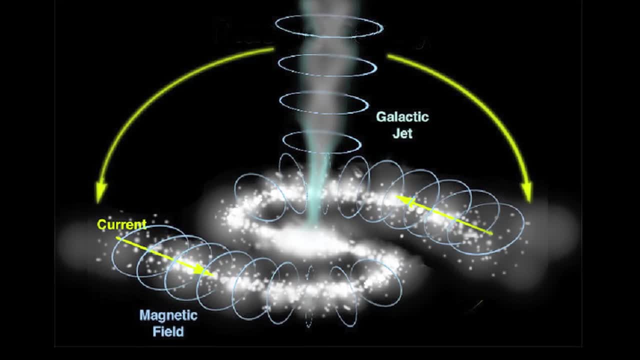 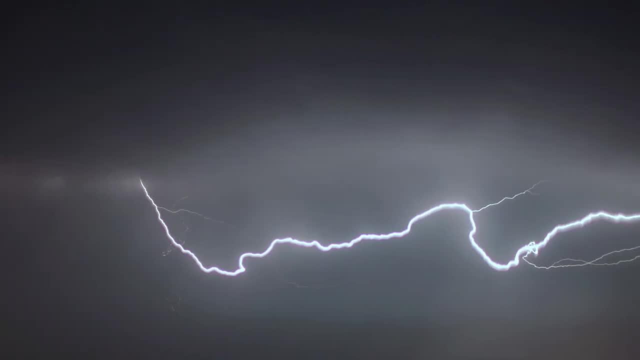 because if this outburst is part of an extended electrical circuit, the fact that it is thin is for the same reason that a lightning bolt is thin and extends over kilometers at the same thickness. And this is what we observe with these jets originating from galaxies. 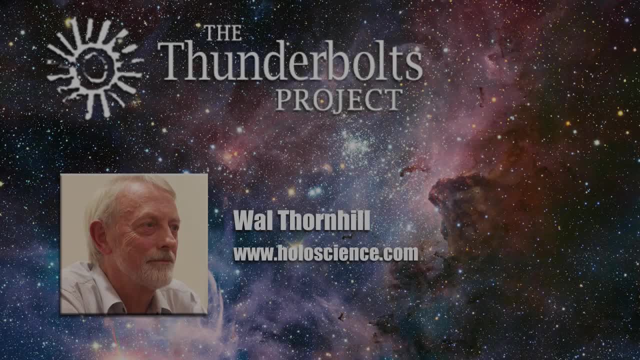 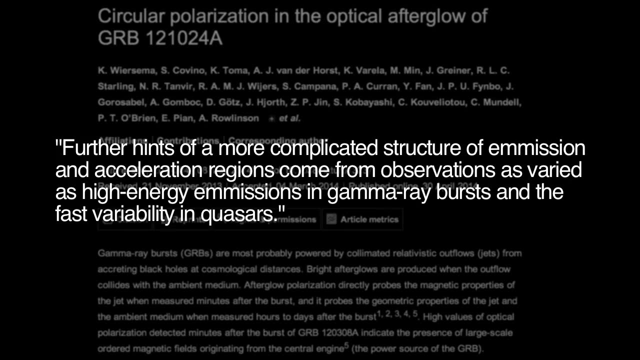 and from supernova outbursts and so on. At the end of the paper in Nature it says: "further hints of a more complicated structure, a structure of emission and acceleration regions, come from observations as varied as high-energy emission in gamma-ray bursts. 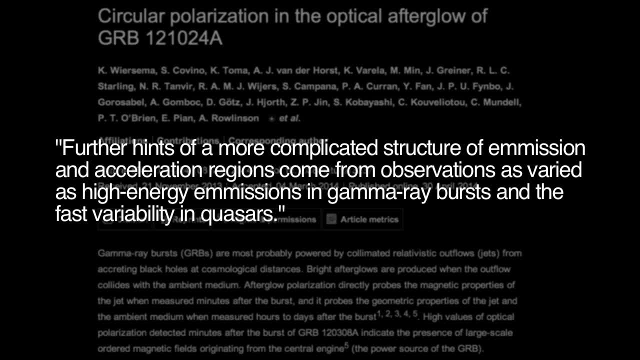 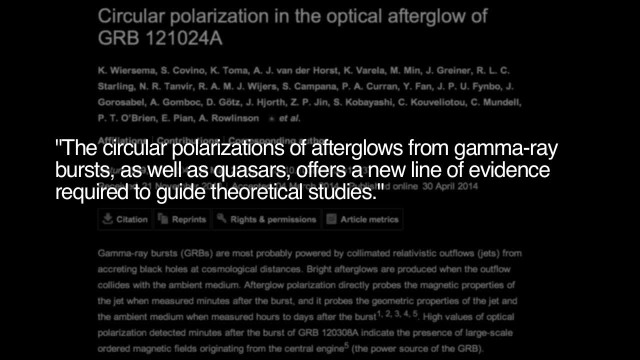 and the fast variability of high-energy emissions in quasars. The circular polarization of afterglows from gamma-ray bursts as well as quasars offers a new line of evidence required to guide theoretical studies". The first thing we have to do is get the concepts in place. 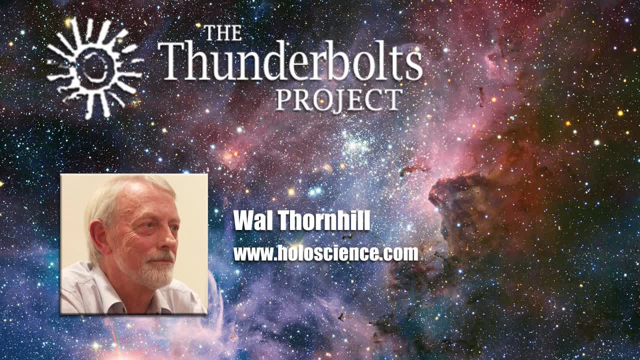 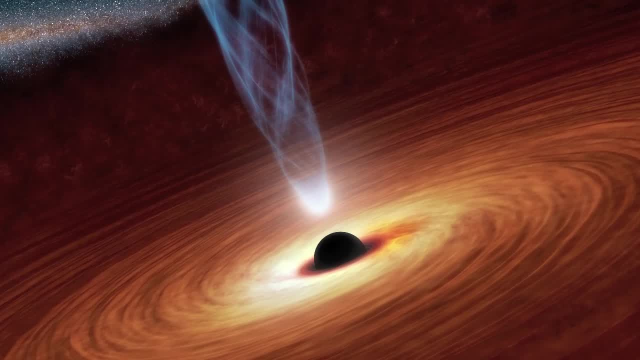 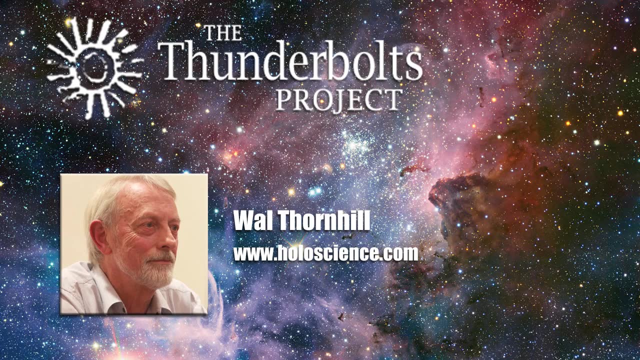 so that the theory can actually work. And this is not going to happen. while we have artifacts like imaginary black holes and quasar activity and active galactic nuclei being driven by super-collapsed matter. The last sentence in the Science News Report says: "extreme shocks like the ones in the gamma-ray burst afterglows.